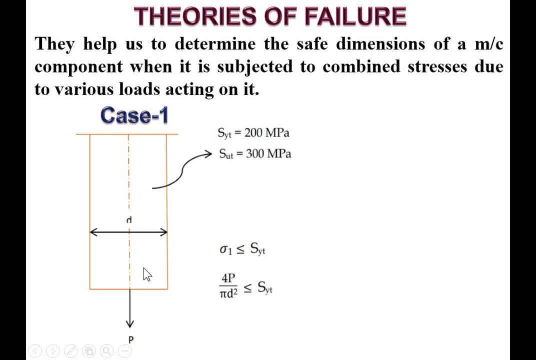 it is very simple to design the machine component. If you know the yield stresses in the tensile stresses it is equal to load upon area and load. you know that p dividable by area stress is equal to load divided by area. So load. you know that p divided by area. So if it's 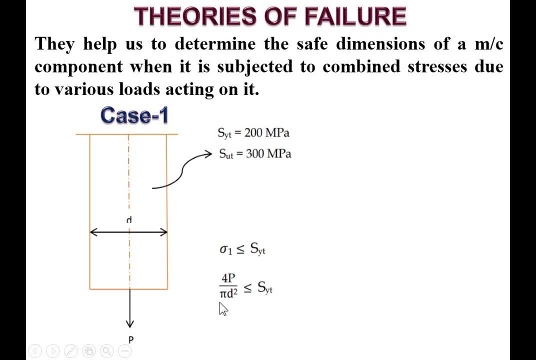 load upon area. stress is equal to area And load. you know that. p divided by area. So if it's it is circular cross section, then it is pi by 4 d square, and that should be equate with the yield strength and so that you can find the diameter of the machine component, if you know. 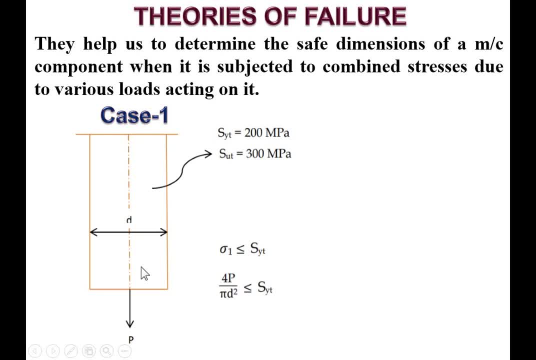 that the value of load. So it is very simple in case number one. Now try to understand the case number two. The same cylindrical shaft is now subjected to the axial load as well as the twisting moment. So at that time it is a little bit difficult to find the value of the diameter. 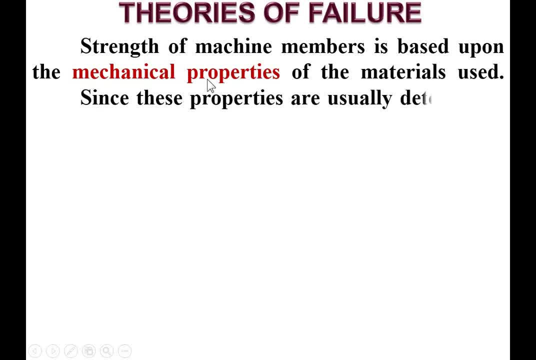 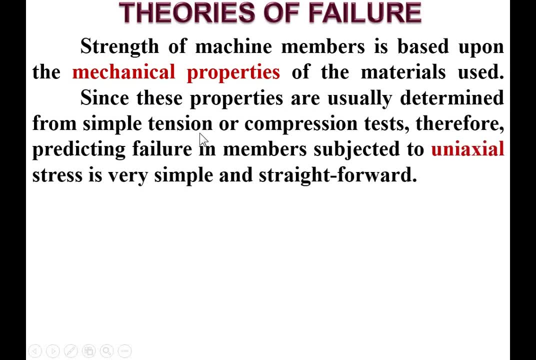 So the strength of the machine members is based upon the mechanical properties of the materials used, Since these properties are usually determined from the simple tension test or the compression test. Therefore, predicting failure in members subjected to uniaxial stress is very simple and straightforward. 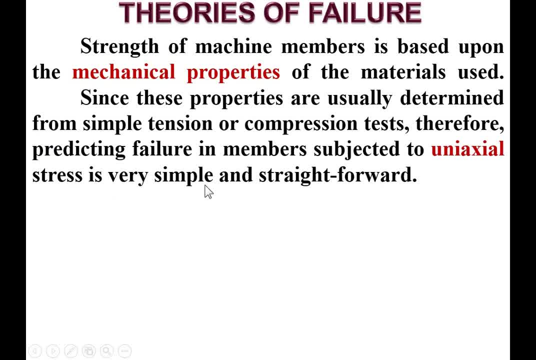 And that we have seen in the earlier slide, or case number one. But the problem of predicting failure stresses for members subjected to biaxial or triaxial stresses is much more complicated and that we have seen in earlier slide, or case number two. So various theories of failures: 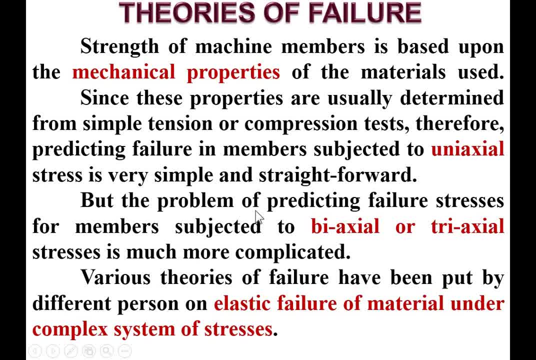 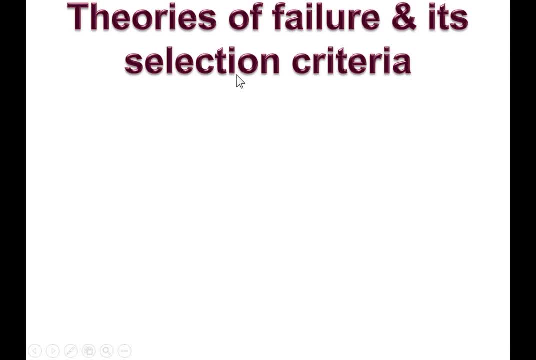 have been put by different person in case of biaxial or triaxial stresses On elastic failure material under complex system of stresses, And so that we should learn the different theories of failures and its selection criteria. So first, maximum shear stress theory that 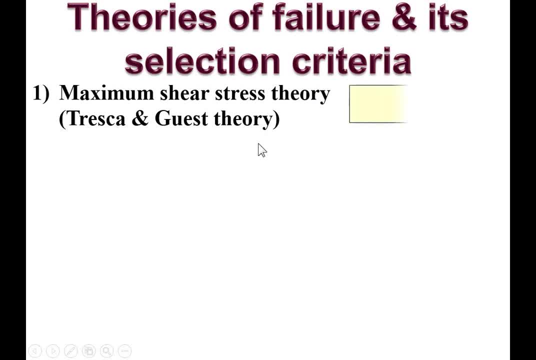 is sometimes known as Tresca and gas theory, And that is suitable for the ductile material. Second theory is the maximum distortion energy theory. that is sometimes known as one-micellar and hanky theory, But generally it is called as one-micellar theory only, And that is. 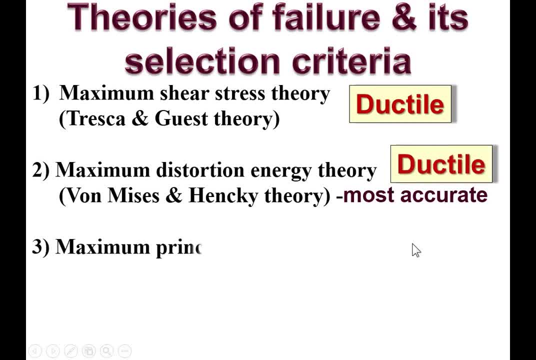 most accurate for the ductile material. Third one: maximum principle, or sometimes it is called as maximum normal stress theory. That is also known as Rankine theory And that is suitable for the brittle material. And fourth one, Coulomb-Moore's theory, that is also used for the brittle material. 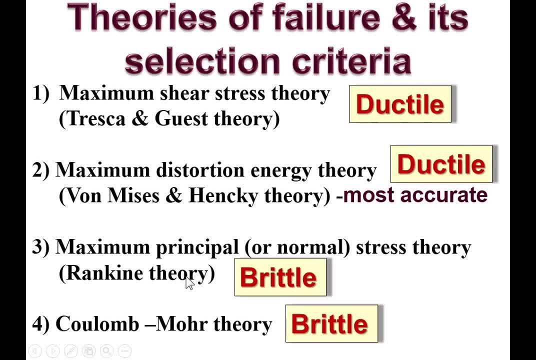 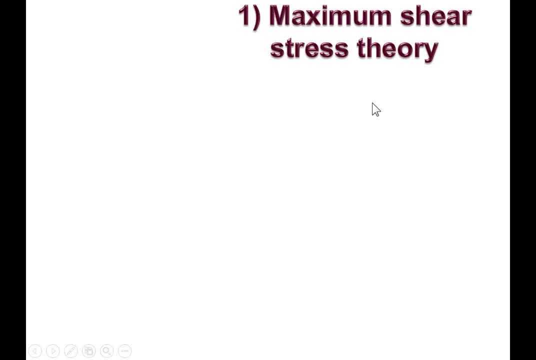 So this all theory we are going to discuss one by one in detail in this session. So let's start from the first one, maximum shear stress theory. So first statement. So it states that the failure of the mechanical component subjected to biaxial or triaxial 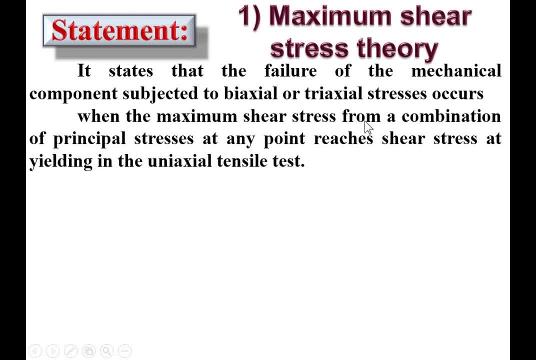 stresses occurs when the maximum shear stress from a combination of principle stresses at point reaches shear stress at yielding in the uniaxial tensile stress. so these two lines are the condition for the maximum shear stress theory and this one is the conclusion. so simply you can say if the machine component is subjected to: 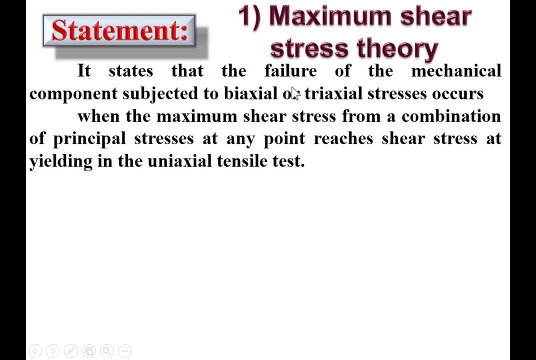 biaxial or triaxial stresses. it will fail when the maximum shear stress at any point reaches the shear stress in the uniaxial tensile test. so failures occurs when that maximum shear stress is greater than the stress at yielding in the uniaxial tensile test. so this is the shear stress yielding in the uniaxial 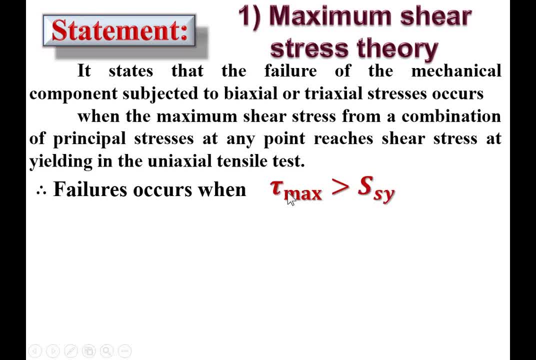 tensile test. so if your tau max is greater than shear stress in the uniaxial tensile test, then this problem should be �m詭. material will fail. So you can say tau max is greater than or equal to 0.5 into sYt, where sYt: 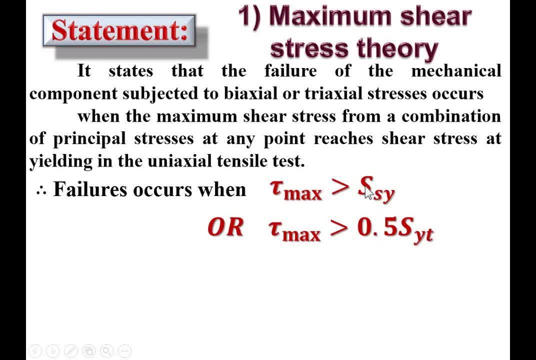 is the yield strength in tensile. So you can say yield shear stress that is always half of the yield tensile strength. So for a safety your tau maximum is up to sSy. If it is more than sSy then the material will fail And if the factor of safety is given to you, 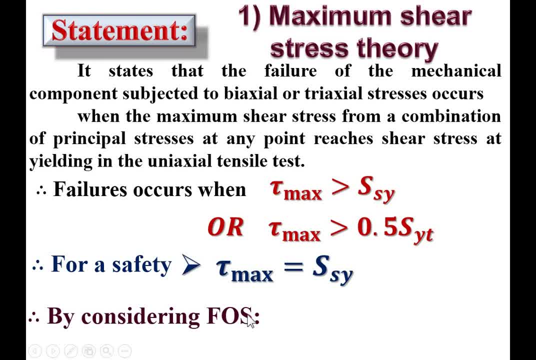 then you have to consider the factor of safety also. So at that time your tau max is equal to sSy upon NF. So NF is your factor of safety. So you know that sSy is equal to 0.5 sYt by. 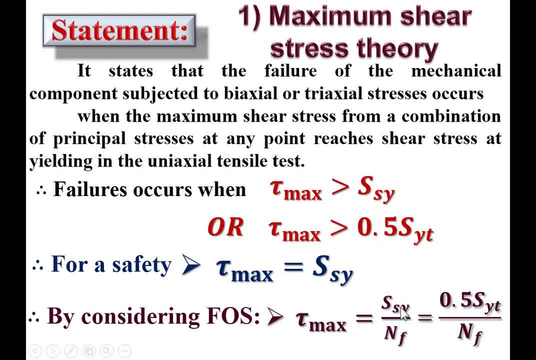 NF. So if the shear stress is given to you in case of uniaxial tensile test, then you can be able to measure the factor of safety, which is 0.5. as to the units of значlished can use this equation. If yield strength in tensile is given to you, then you can use 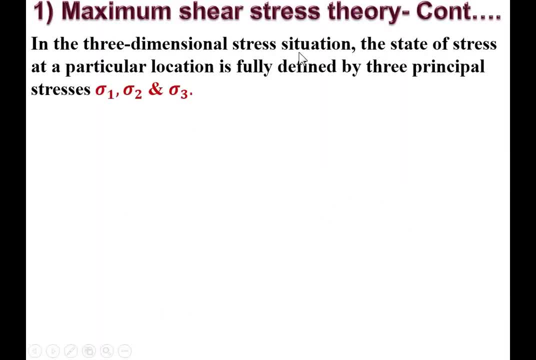 this equation. So in the three-dimensional stress situation, the state of stress at a particular location is fully defined by three principal stresses: sigma 1, sigma 2 and sigma 3.. So the extreme value of shear stress: tau12, tau13 and tau23.. If we assume that, 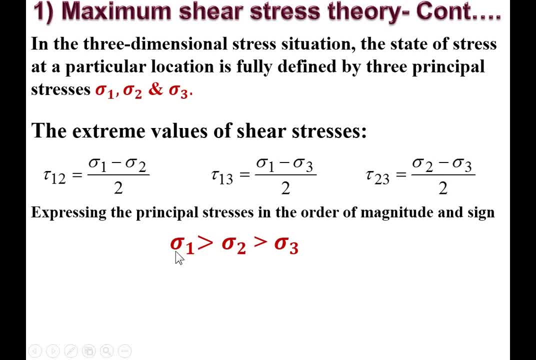 the relation between these three principal stresses is like that sigma 1 is greater than sigma 2 is greater than sigma 3, so at that time you can say: sigma 1 is a major principal stress and sigma 3 is the minor principal stress. So here you can say the maximum shear. 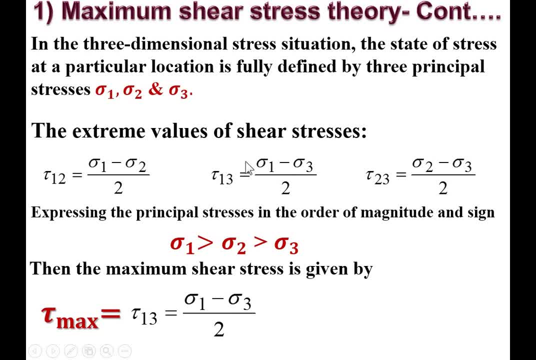 stress, that is tau13.. So tau13 will be the maximum out of these three different shear stresses. So you can say tau max, that is tau13 is exactly tau i over tau x 3, that is sigma 1 minus sigma 3 by 2.. So you can say sigma 1, that is the S y t that. 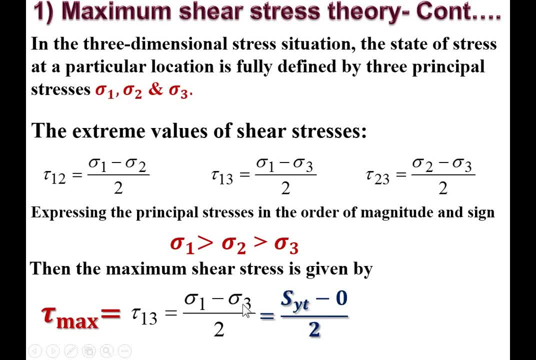 means yield stress in tensile, and sigma 3 is 0 in case of two-dimensional stresses. So if you simplify then you will get S y t by 2 and that we have discussed in earlier slide, that tau maximum is equal to S y t by 2.. So you can say it is 0.5 S y t, So that 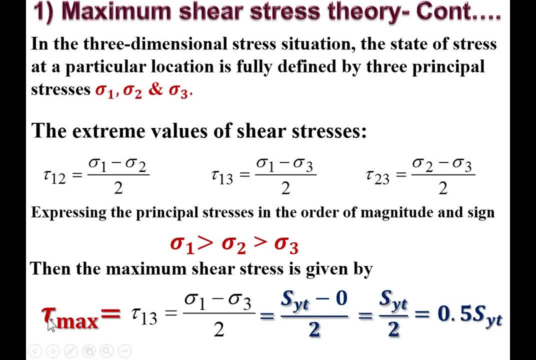 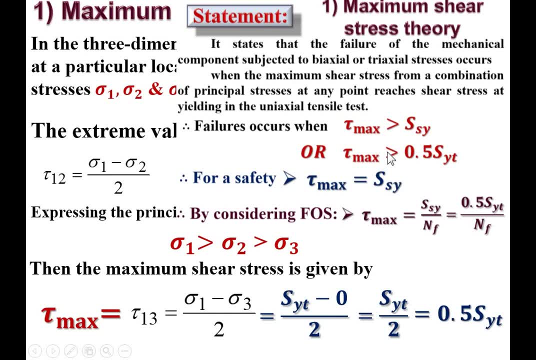 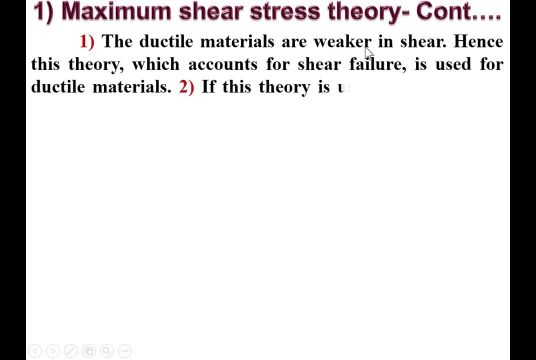 is the mathematical statement of maximum shear stress theory. tau maximum is equal to 0.5 S y, t, So that we have discussed in earlier slide Now the selection criteria. The ductile materials are weaker in shear always, and hence these. 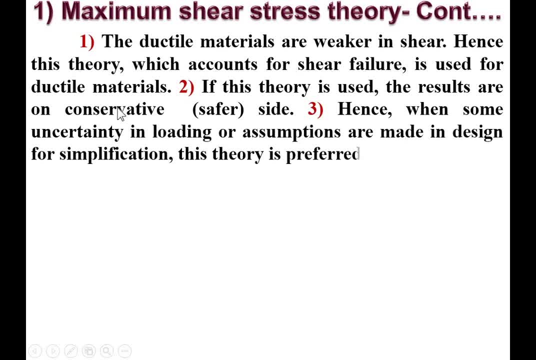 theory which accounts for shear failure is used for the ductile materials. If this theory is used, the results are on conservative side. that means much more safer side. Hence, when some uncertainty in loading or assumptions are made in design for simplification, this 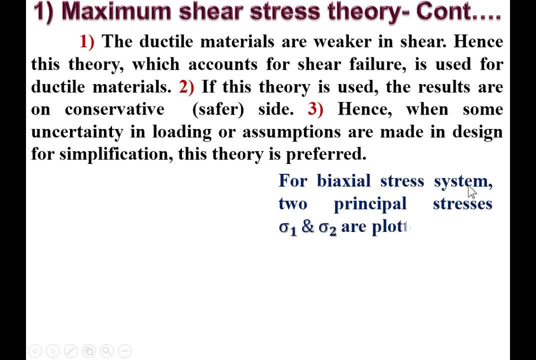 theory is preferred For biaxial stress system. two principal stresses, sigma 1 and sigma 2, are plotted on x and y axis as shown in figure. So here you can see sigma 1 on x axis and sigma 2 on the y axis, and sigma 1 and sigma 2 are the major. 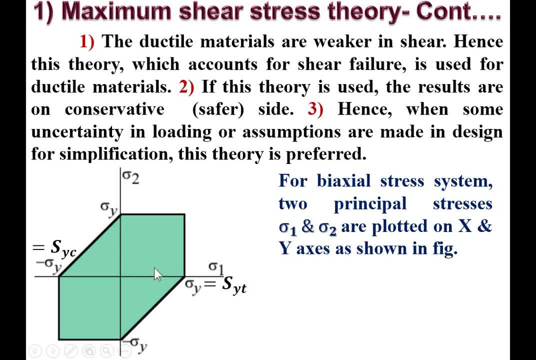 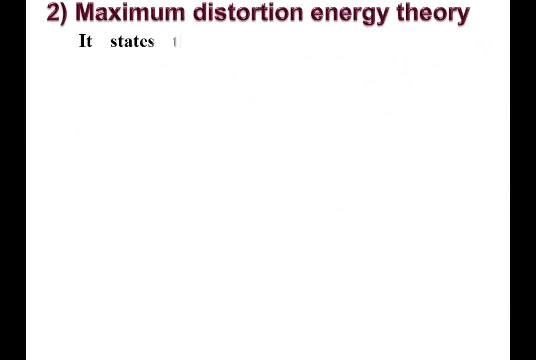 principal stress and minor principal stress respectively, So that this zone is called as the safer zone. So you can say the green color is the safe zone according to this. So in this case, sigma 1 on x axis is considered to be safe zone. 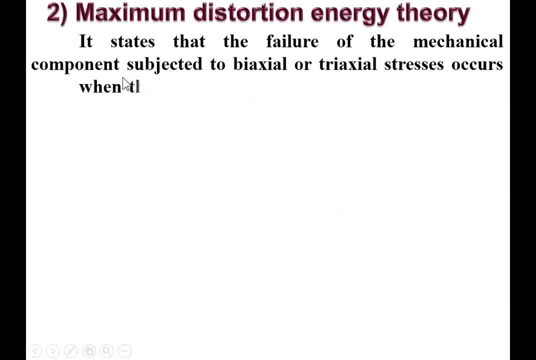 Now second one: maximum distortion energy theory. So first try to understand this statement. So it states that the failure of the mechanical component subjected to biaxial or triaxial stresses occurs when the distortion energy per unit volume at any point in a component. 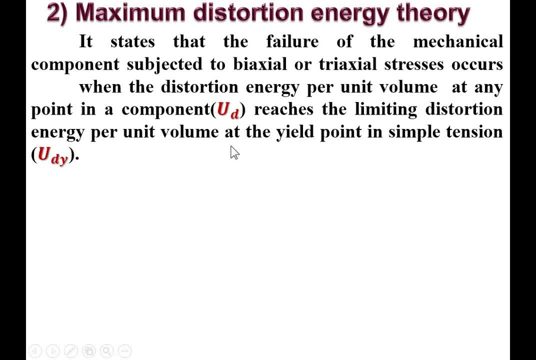 reaches the limiting distortion energy per unit volume, The disparity in the distortion of the component is greater than the threshold value of the component. So this means that the distortion energy per unit volume at any point in a component unit volume at the yield point in simple tension test. 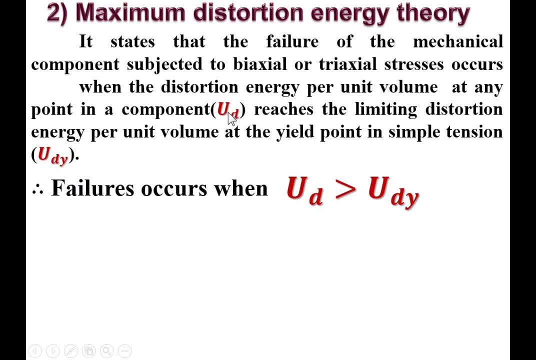 So failures occurs when Ud that is greater than Udy, where Ud is what? once again the distortion energy per unit volume and Udy that is the limiting distortion energy per unit volume in a simple tension test. So for the safety, so that is actually derived equation. 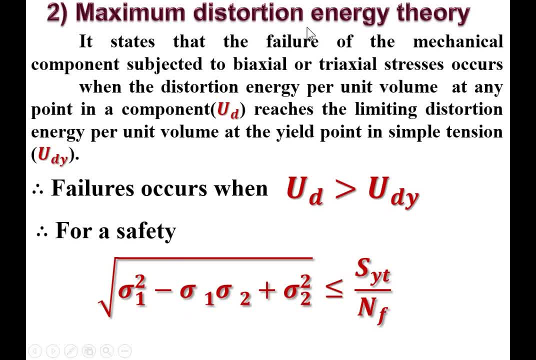 So directly. you have to remember, for a safety in case of maximum distortion, energy theory, square root of sigma1 square minus sigma1 into sigma2 plus sigma2 square, that should be less than or equal to Syt upon nf, where sigma1 and sigma2 are the major principal. 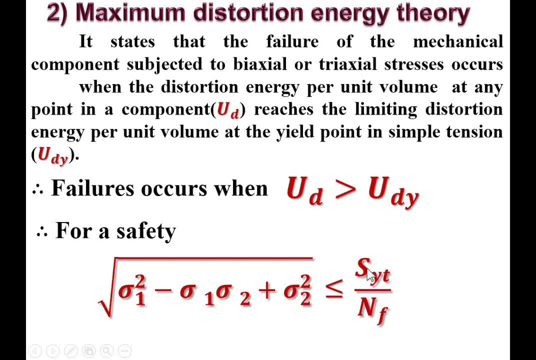 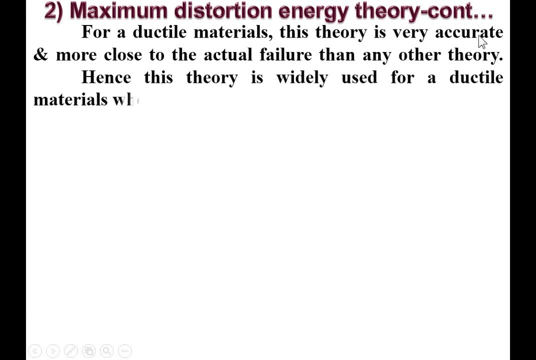 stress and minor principal stress respectively. Syt is the yield stress Intensile and nf that is the factor of safety, So the selection criteria for a ductile materials. this theory is very accurate and more close to the actual failure than any other theory. 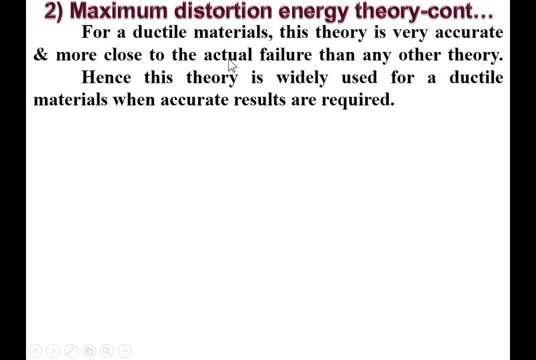 So if you compare this maximum distortion energy theory with the maximum shear stress theory, then maximum distortion energy theory will give you very accurate result. Hence this theory is widely used for a ductile materials. when accurate results are required, This is the safer zone according to the maximum distortion energy theory. 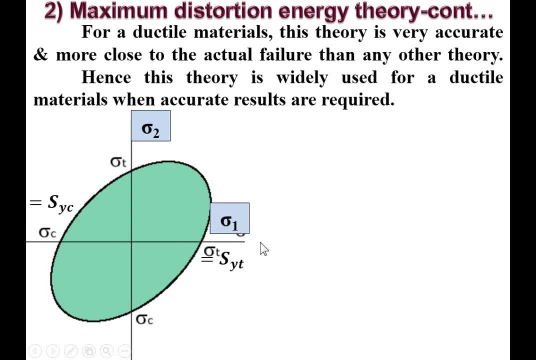 So if we plot major principal stress on the x axis and minor principal stress on the y axis, then this is the safe zone according to maximum distortion energy theory. Now If we compare with the maximum shear stress theory, then this is the safe zone by maximum. 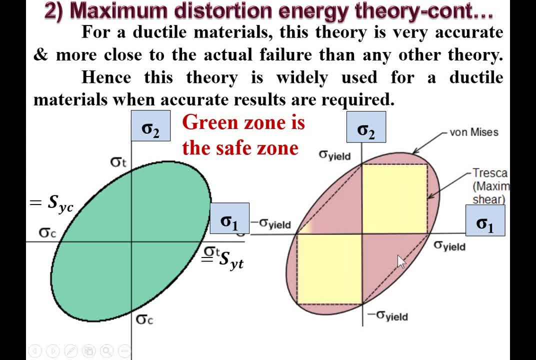 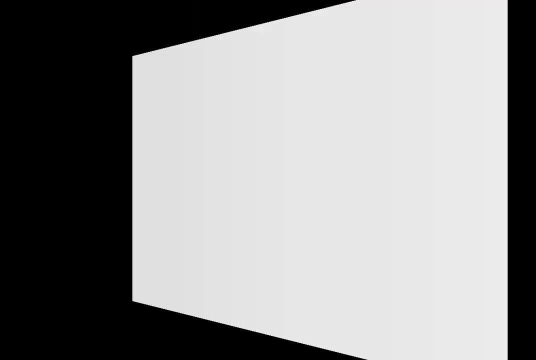 shear stress theory. So if you highlight over here with the different color, then this yellow shade that is according to the maximum shear stress theory, that is also known as Traskas theory, and this pink color is according to the von Mises theory, That means maximum distortion energy theory. 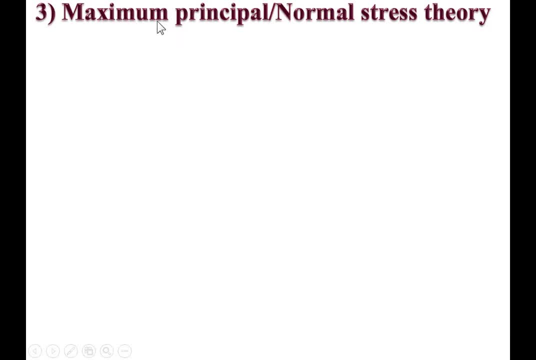 Now the third one: maximum principal stress theory, or you can say maximum normal stress theory. So the following is the momentum- trying to get an idea upfor buying these structures to bliss our content of BIM. So statement-: The failure or yielding occurs at a point in a member when the maximum principal 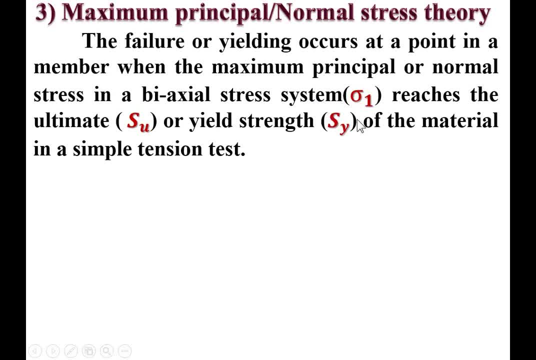 or normal stress in a biaxial stress system reaches the ultimate or yield strength of the material in a simple tension test. So the condition of failure for the machine component is sigma1, greater than or equal to sy or su. So sigma1, that means what?